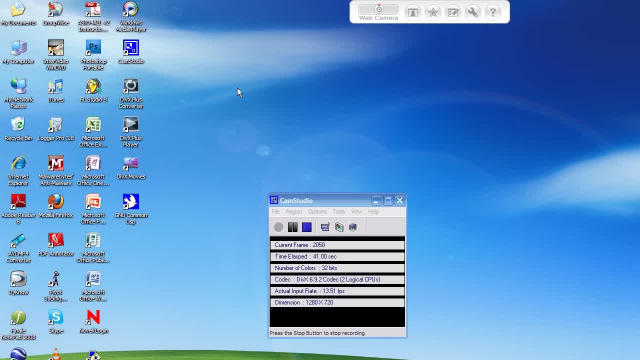 So I'm going to start off by showing you guys how to get- let's go- common list for Windows. So if you're on Mac or Linux or Unix or any of those systems, I'm not sure how to help you. You could probably just look up. 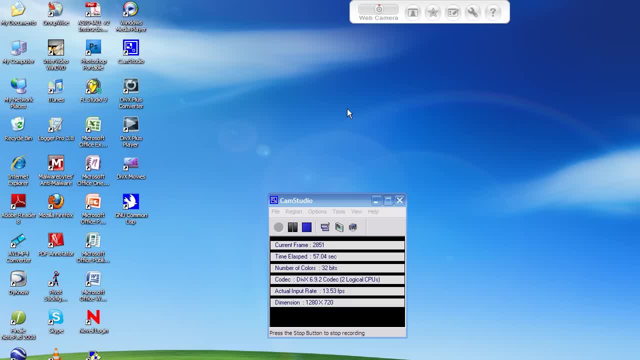 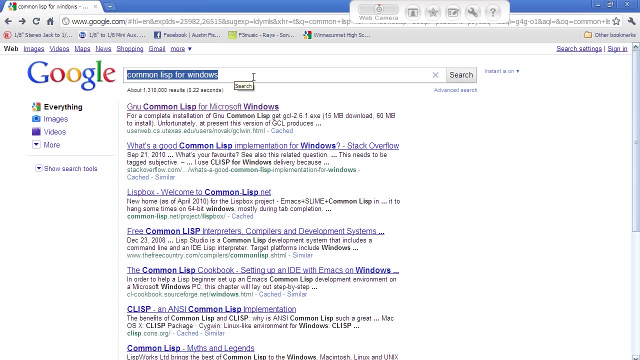 common list for any of your operating systems and you'll probably find what's called an interpreter for it, But I'm going to show you how to get it for Windows. So what I did is I just googled common list for Windows and I got this right here- GNU common list for Microsoft Windows- And then I just clicked on this and downloaded. 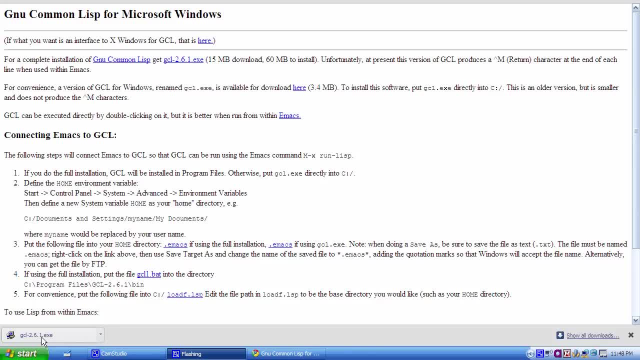 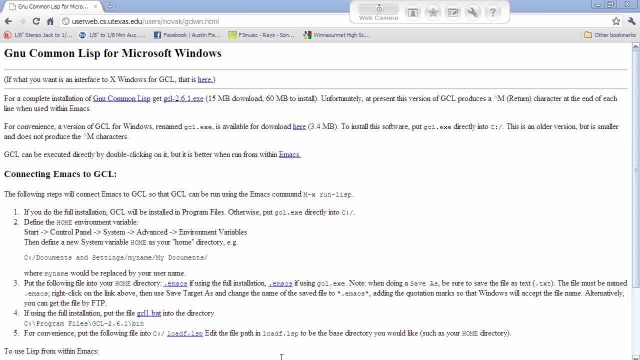 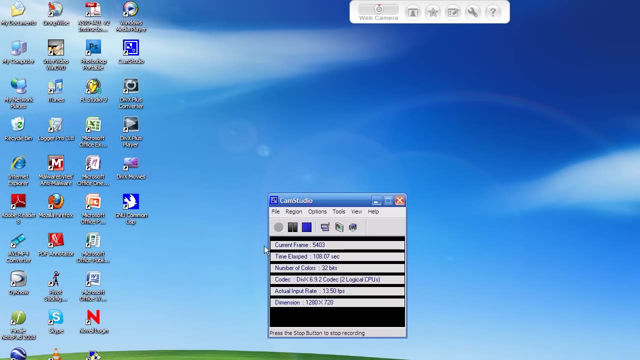 the file. It's right here: GCL 2.6.1.. That's the current version, the current, most recent version. It might be different at the time that you find it, But anyway, this is what I got. You can really find or use any that you find out there, as long as it's a LISP, What's it called? Interpreter or whatever the fuck it is. 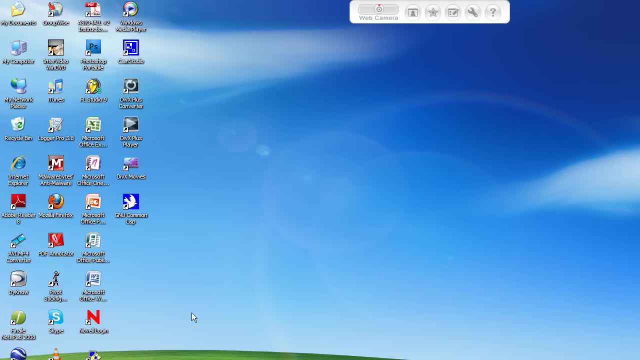 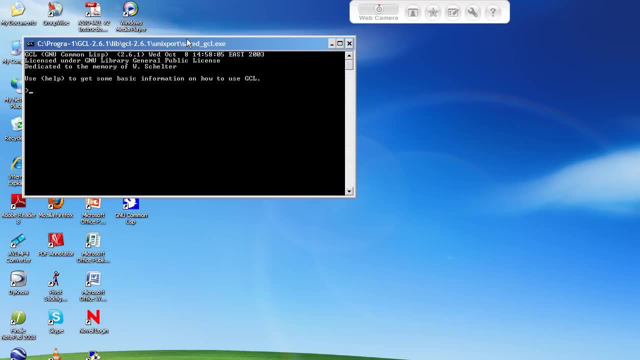 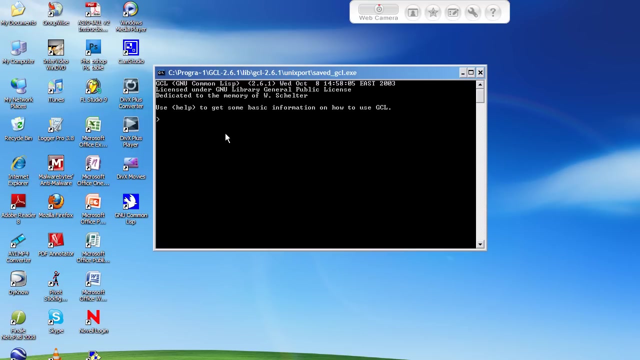 Oh, anyway, let me move that up here. So what you're going to do is, after you've done installing it and everything, you're just going to open up the file here and it's going to bring up this window which looks like command prompt, because it basically is command prompt. Now in here we're going to start out with the very, very basics, and that is adding and subtracting, The most basic thing you can do in LISP. Now, in LISP, everything is a list, and so that means everything is enclosed within parentheses. 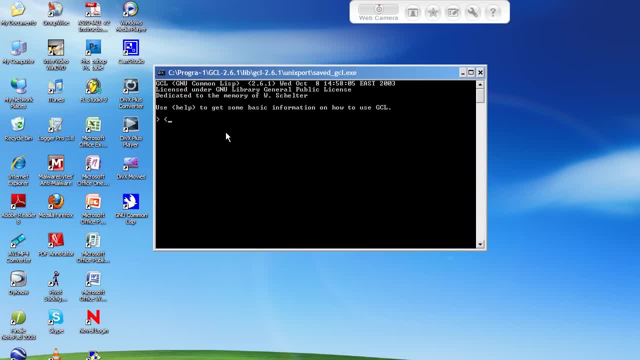 So every line of code you have will start out with an opening parenthesis. It will look a lot like the arrow here, but it's an opening parenthesis- And then you have whatever code you want and then an ending parenthesis. So, to start out, LISP, instead of doing something like 1 plus 1, what it's going to do is you do the plus first and then you list all the numbers you want to add together afterwards. So I'm going to add 1, 1, 1, 1, 1.. 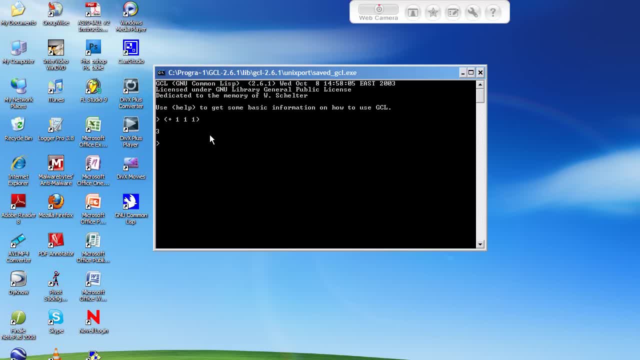 one, it's gonna give me three. now you can do the same thing for subtract. I'll do four and three, which is one, and I'm pretty sure you can do the same thing for multiply and divide and so forth. just gonna give examples for each, so ten. 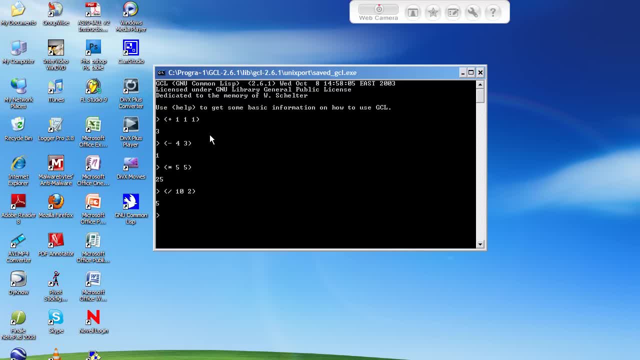 divided by two. now let me just check this one thing: if we divide 9 by 4 or 2, that's okay. okay. so, and lisp, at least with this interpreter, a lot of interpreters will give you different results sometimes. if you divide by something that's not a whole number, it's gonna give you a lot of different. 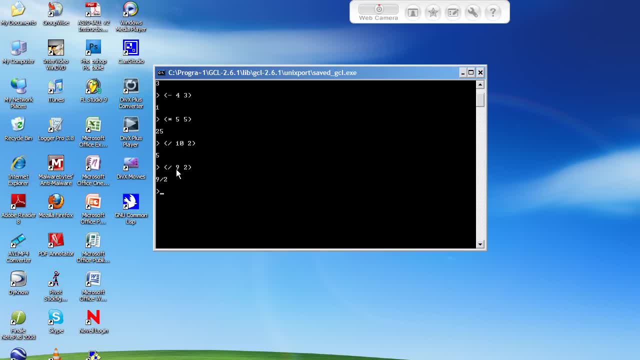 results. sometimes we'll just give you the rounded numbers, so that's in this case. it would give me five, because nine divided by two is four point five rounded up would be five. either that, or it might just kick off the decimal and give you four, or in this: 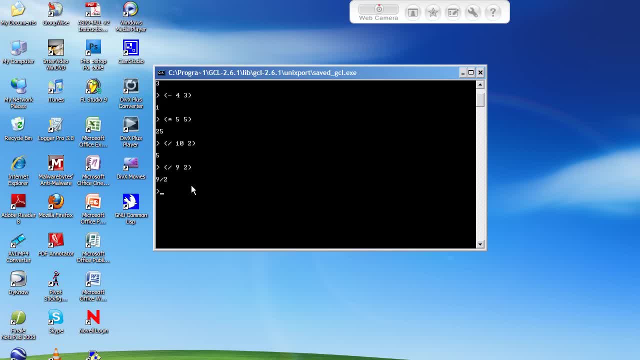 case, we'll just give you the fraction, which is 9 over 2, which is- let me do the math, oh my god, I feel like an idiot. four and one half- I could have done that before. okay, I'm in geometry honors and I really had to do that. whatever. 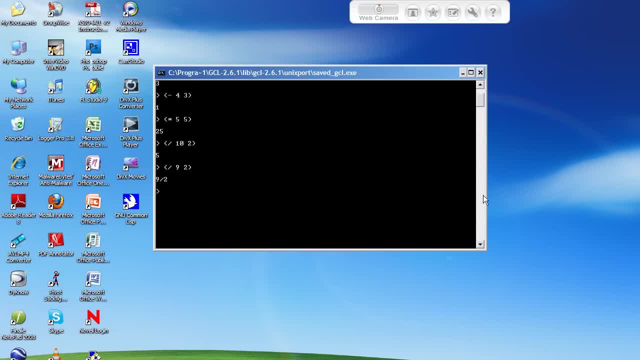 but so that's pretty much the basics of math in lisp. I'm only doing these tutorials, really, because I found that there's no like real tutorials about lisp on YouTube, so I'm hoping to get this out there because this feels like a really amazing programming language. I'm surprised nobody decided to do one before, so. 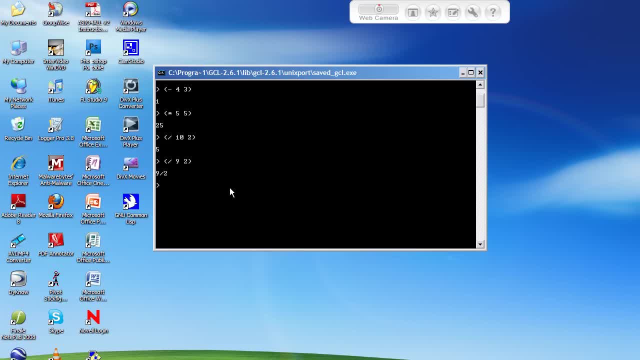 anyway, that's, that's the end for this tutorial. what am I talking about? I can go into way more detail, so here it is. what you can basically do is say you want to add the product of two products, so say: add 5 times 5, 5 with 3 plus 6. the way you do that is: add that.